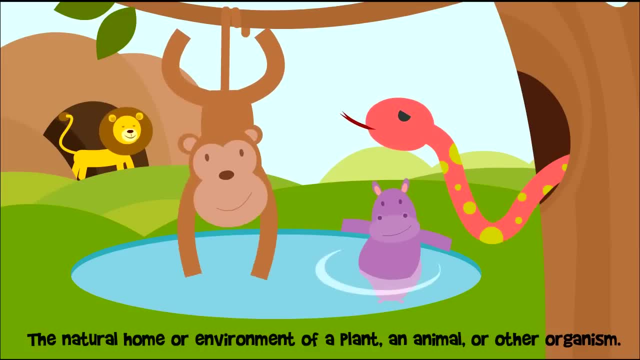 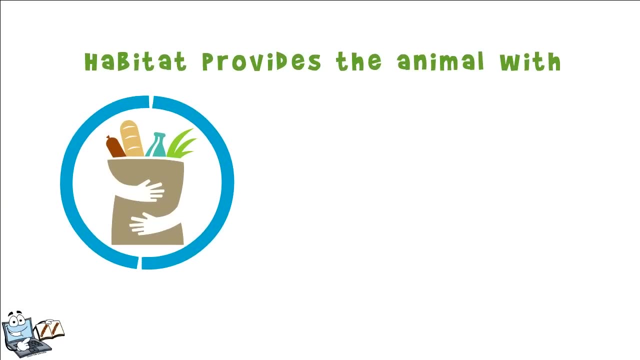 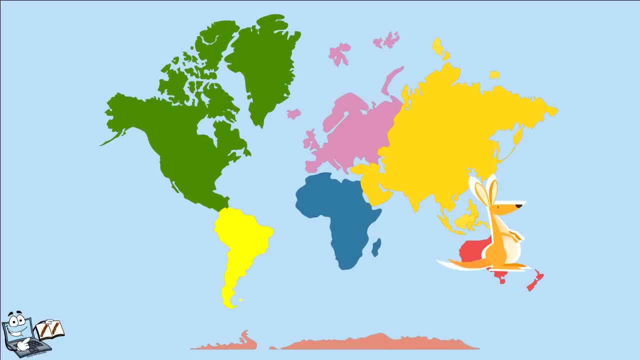 the natural home or environment of a plant, an animal or other organism. Habitats provide the animal with food, water and a place to live. There are many different types of habitats around the world, from grasslands to forests and from big mountain. 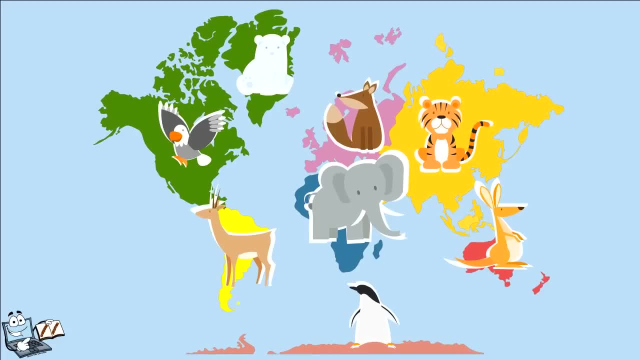 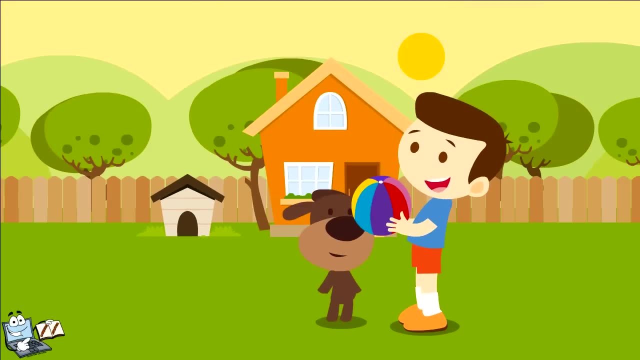 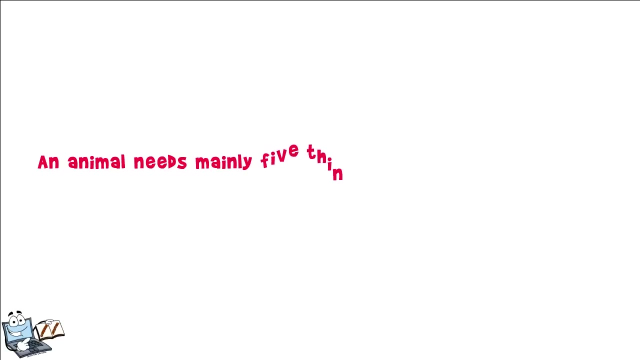 slopes to large deserts. Different habitats are shelter to different animals. When we speak about an animal's or a plant's house, it is more like a neighborhood than a home. An animal needs mainly five things to survive in its habitat: Food, water, air, shelter and a place. 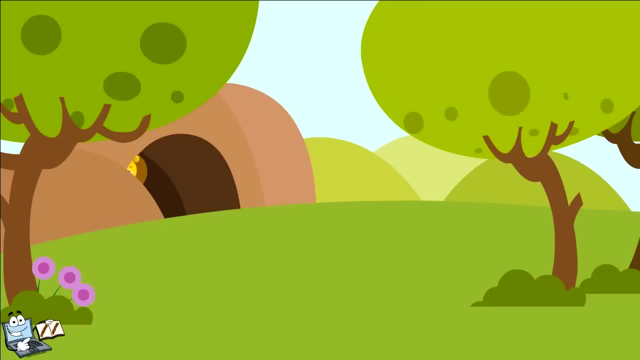 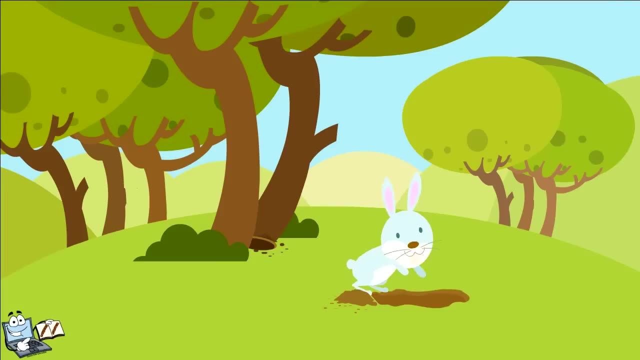 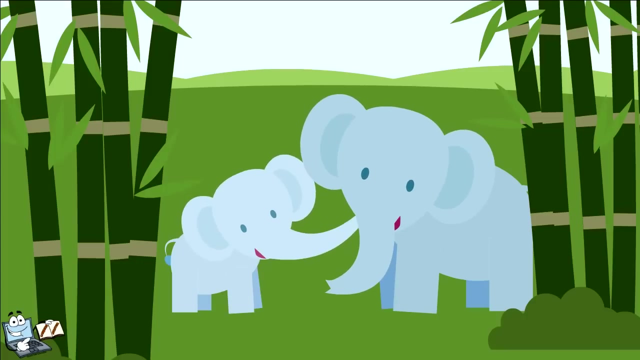 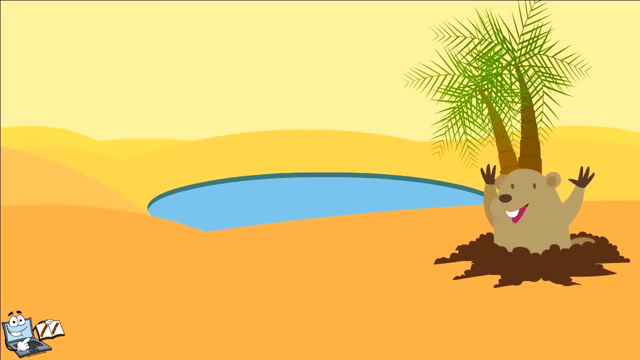 to raise its young ones. Different animals require different amounts of space to live in. Habitats can be large like a forest, or they can be small like a burrow. Some big animals defend a huge territory or roam over a large area. Some other animals need only a small amount of space and can 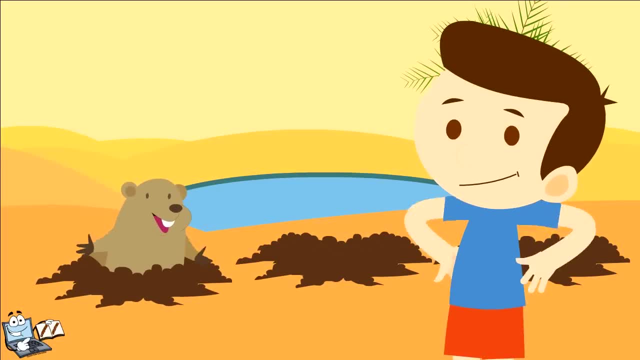 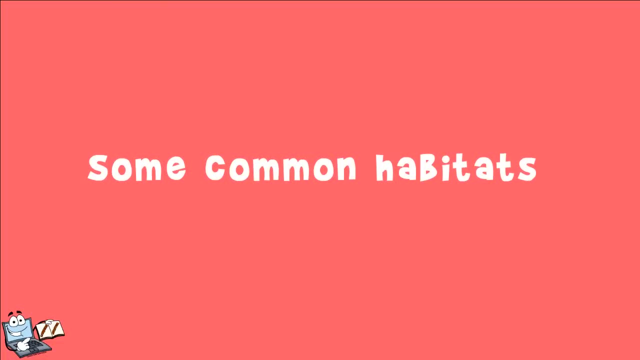 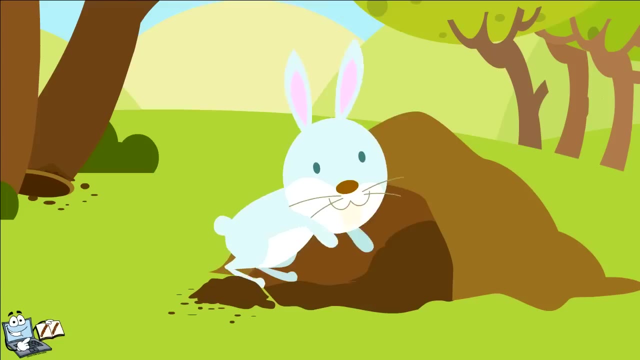 put up with neighbors that live close by. Oh, you are very much interested in learning this Great. There are some common habitats where animals live. You can place this chart in your room so that you remember it. Now you know that different animals 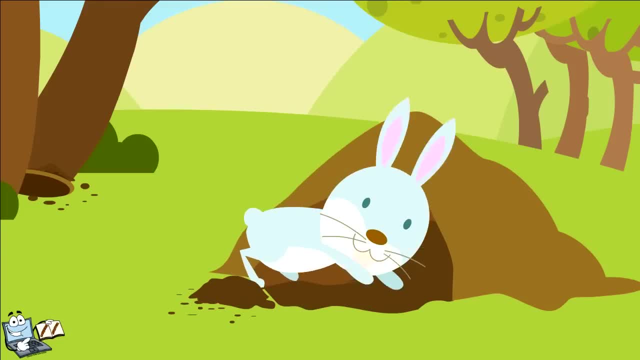 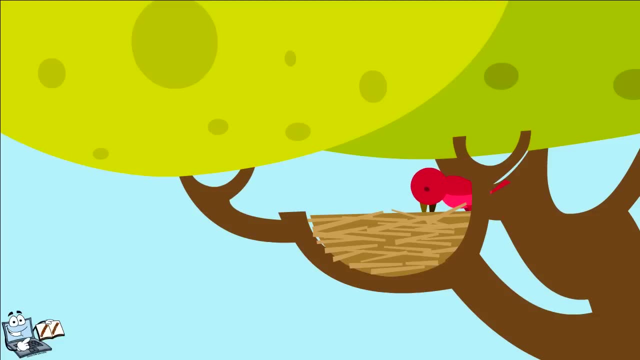 live in different types of houses. Some animals are so clever that they make their own homes. Here are the common names of animal homes: Homes of Birds. A bird's home is called a nest. Most of the birds make nests from grass, leaves, fur, lichen. 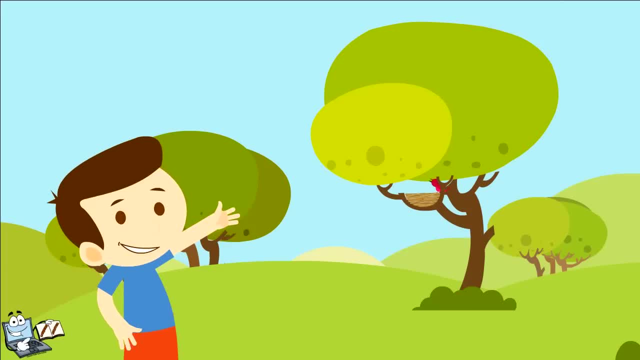 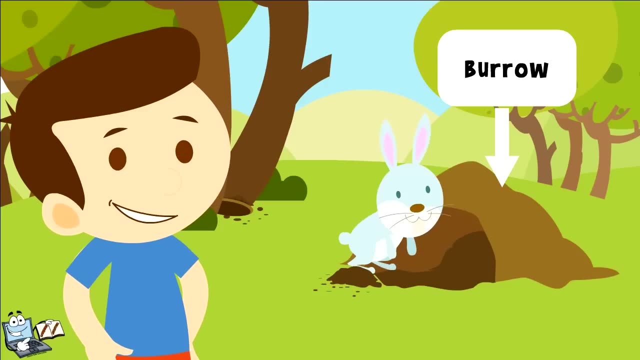 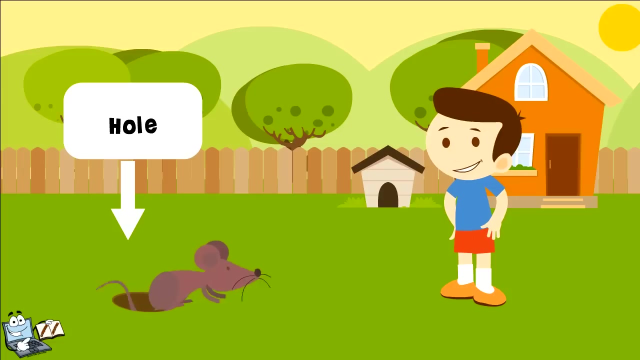 and mud, or from paper, plastic and yarn, The Home of a Rabbit. A rabbit's home is called a burrow. Rabbits dig burrows to live in The Home of a Mouse. A mouse lives in a hole. Mice dig holes to live in Home of a Spider.